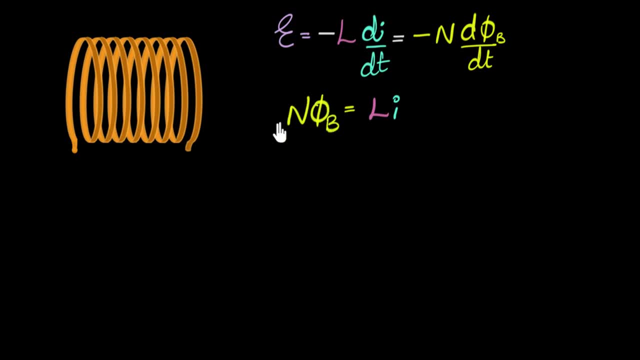 because this is a cool relationship. What is it saying? This represents the total flux through our solenoid, So it's N times flux through each coil. So this is the total flux equals. it's saying that the total flux is proportional to the current. 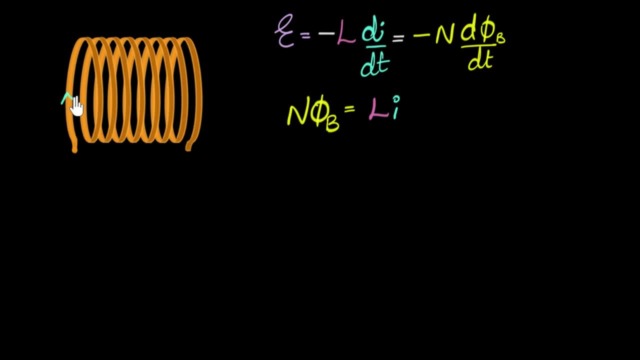 Does that make sense? Of course it makes sense, right, When you pass some current through it, some current I. it's that current that's generating the magnetic field and it's that magnetic field that's causing the flux. So more current gives you more magnetic field. 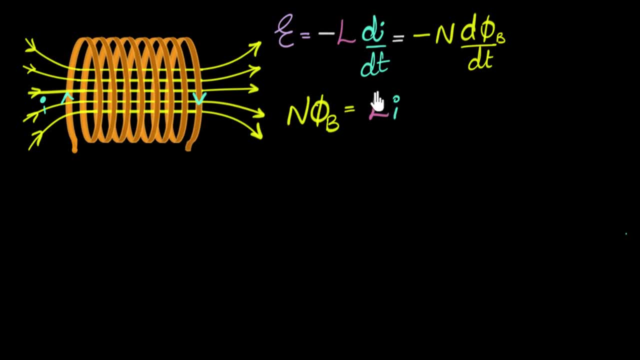 giving you more flux. So it makes perfect sense. And the constant is the self-inductance. And why I like this is because you can do something very cool with it. You can compare this with something we've learned in mechanics: Flux is like momentum. 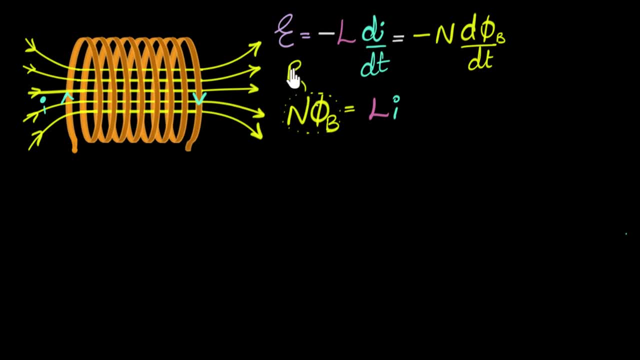 Think about this for a second, okay. Why I like to think of flux as momentum is because in mechanics we've seen that if you want to change momentum of an object, then you have to put a force on it. But when you put a force on it, 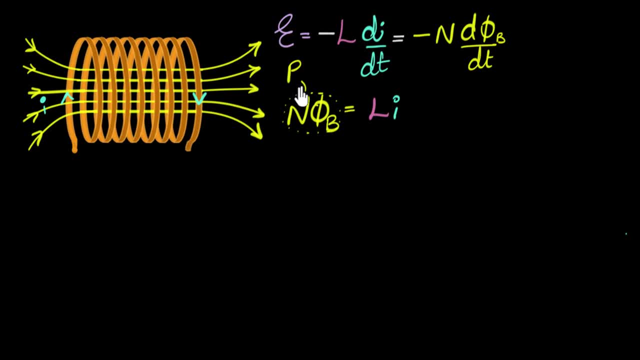 from Newton's third law: it pushes back on you. So that means whenever you try to change momentum of an object, that object will push back on you. It's very similar to what we're seeing over here. We can say: objects hate changes in momentum. 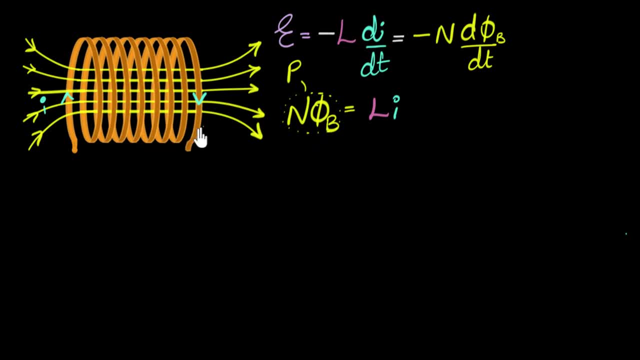 And flux is very similar. Coils hate changes in flux. You try to change the flux, they'll push back on you by inducing an EMF And we've seen the momentum equals mass times, velocity, where mass is their inertia, And similarly self-inductance is the electrical inertia. 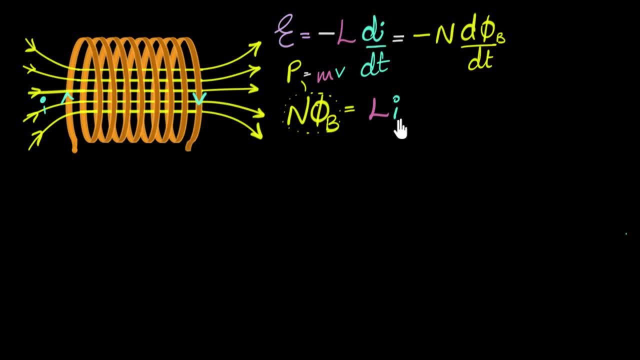 And velocity is the speed at which objects move And you can think of, current is proportional to the speed at which charges are moving. So do you see? a neat relationship exists between the two. Beautiful, isn't it? In fact, you can use the relationship here also. 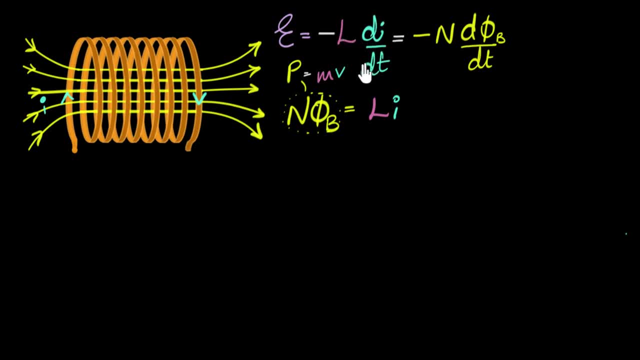 and you get something very similar. Force equals mass times dv over dt, And you can explore that yourself. But anyways, now we can calculate what the self-inductance is. So you can say from this expression: self-inductance of our solenoid equals the total flux. 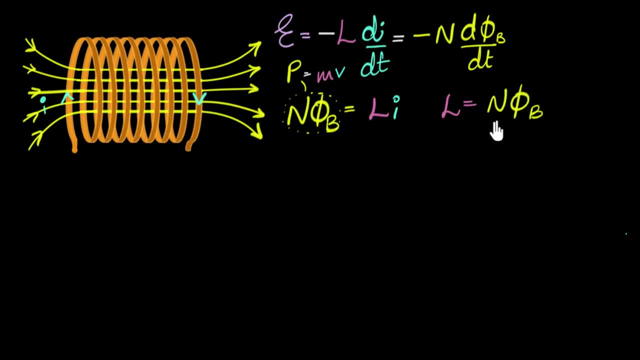 if you pass some current through it, you calculate the total flux and you divide it by the current, Divide by the current. All right, So how do I calculate the total flux? through a solenoid, We know how to calculate the flux through any loop. 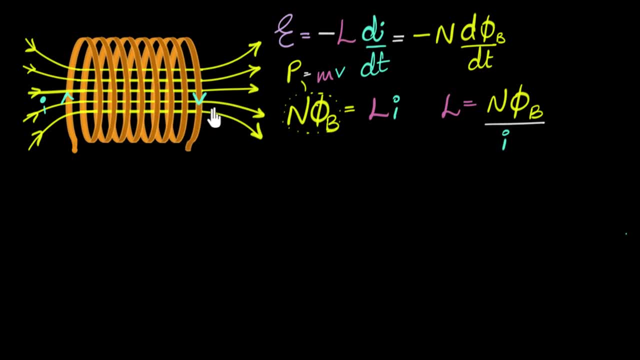 We know the flux equals B times A times cos theta. The theta is the angle between the area vector and the B vector Here. notice the area vector. so if I take one such loop, the area vector would be this way And the magnetic field is also in the same direction. 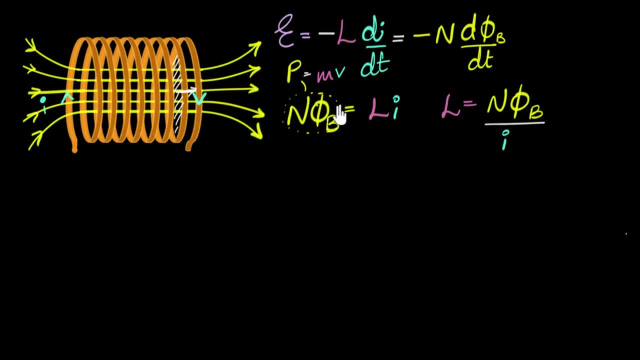 if I assume the field to be uniform And so the flux just becomes B times A, And so if I plug that in, I will get self-inductance equals N times the flux, which is just B, the magnetic field over here. 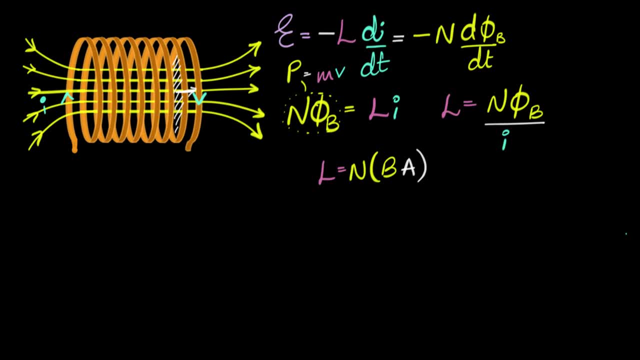 times the area divide by A divide by, I sorry. And now comes the question: what is the magnetic field inside a solenoid? Now, that's something that we have derived before and we can just directly substitute, but my problem is I don't remember that. okay, 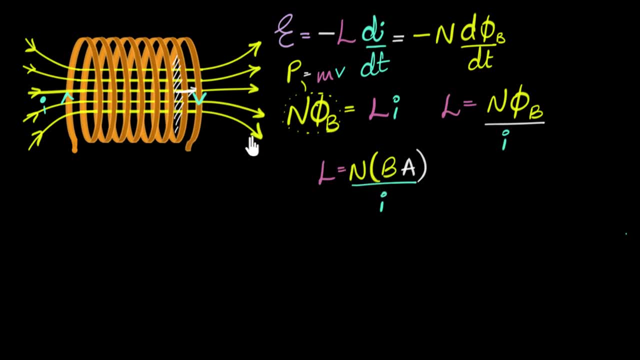 My principle was: I don't remember a lot of formula because physics is not about formula. So what do I do over here? What I like to do is go back and think about how we derived it and quickly make that derivation. And so, if you're like me, 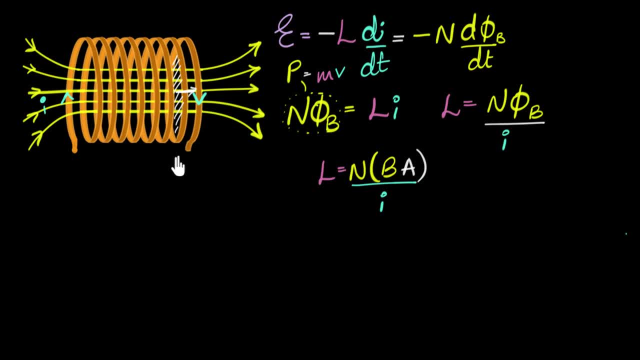 then you would also want to do something like that if you don't remember the formula. But if you do remember the formula, feel free to pause or skip ahead to directly substituting and getting the expression. But if you're like me, then this is what I like to do. 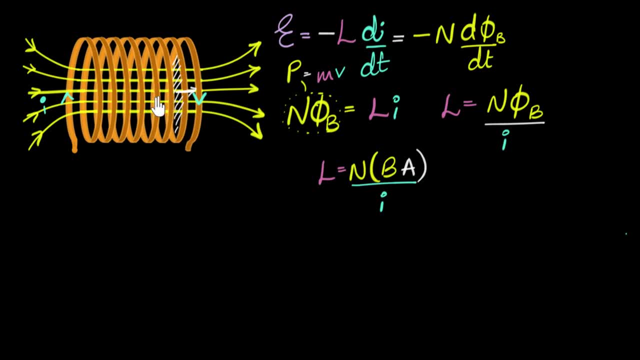 So I go back and ask myself: hey, where did the magnetic field? how did I derive the expression for the magnetic field? So there are two ways to derive it. You use Biot-Savart or you use Ampere's Law. 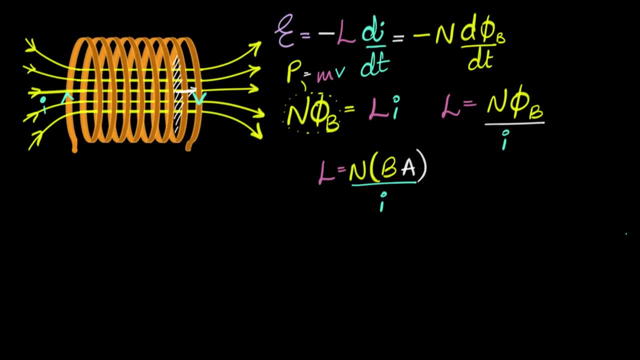 And I remember I use Ampere's Law in some special cases. So I go back and I use Ampere's Law. It says the closed loop integral of B dot DL equals mu naught times. I n closed And so now I have to choose a loop. 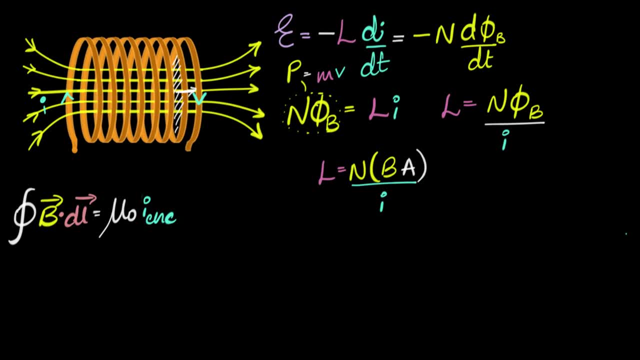 and the clever loop I choose because I have a straight field over here. I remember our Amperian loop is gonna be some kind of a rectangle or a square And when I go around it to calculate B dot DL, notice B dot DL here is zero. 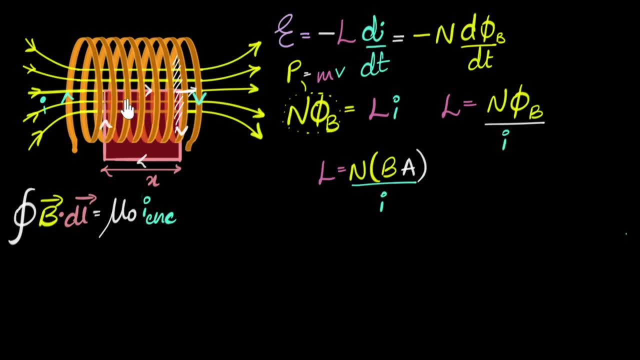 because there's no field outside here And here B and DL are in perpendicular, so B dot DL becomes zero. cos 90 is zero. B dot DL over here is zero, If you can see that same reason, Outside is zero. so the only B dot DL you get is over here. 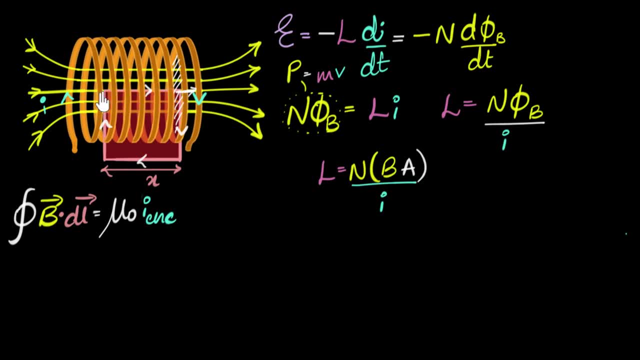 And when you do that, you just get magnetic field B times the length, which is x. So I'm doing a quick derivation, not a complete derivation, If you've done this before. so B times x. so this is how I'm doing my derivation. 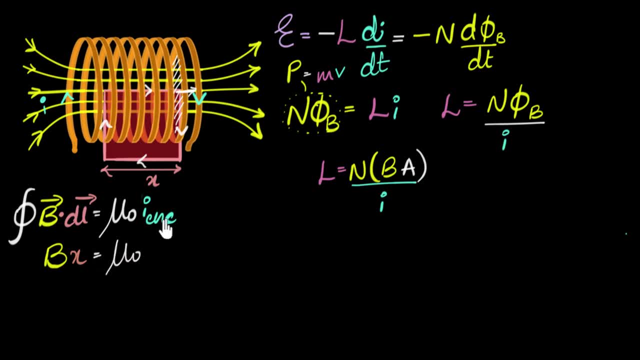 I don't remember the field value at all, So that equals mu naught times I n closed. so that's the total current enclosed by the loop. What is I n closed? That'll be the total number of loops enclosed, n enclosed, multiplied by the current through each loop. 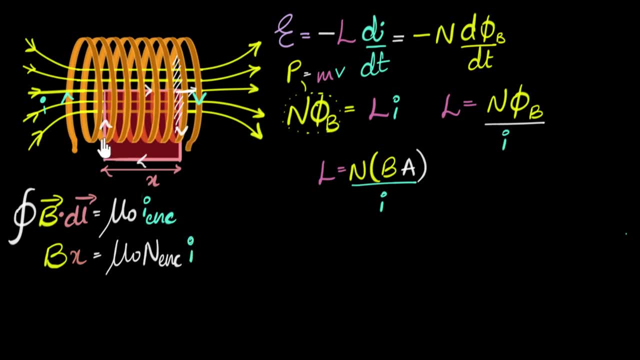 that is just I, And so now I ask you how many loops are enclosed? What's the ratio for that? So I know that if I take the total length of the solenoid to be, say, L, and let's say the total number of loops is n, 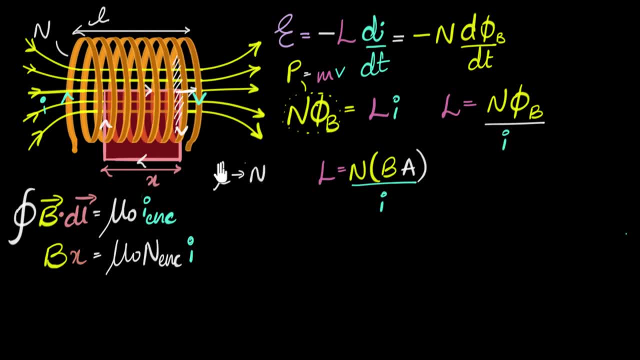 then I know L has n number of loops, so the length x has how many loops. So it's gonna be nx by L, So I can just substitute this as nx over L. so this is nx over L, and there we go. 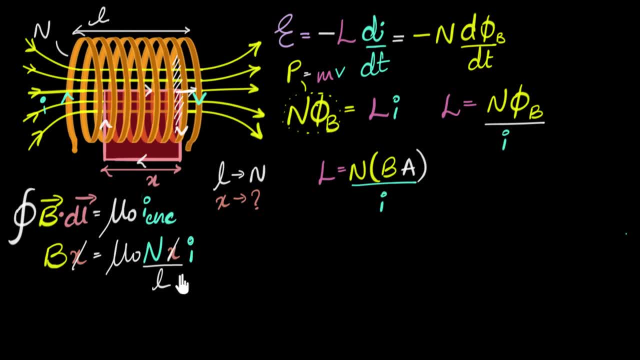 X cancels out, And that's the expression for the magnetic field, So you don't have to remember things. So what I like to do is remember basic fundamental rules like Ampere's Law, Biot-Savart Law, Faraday's Law. 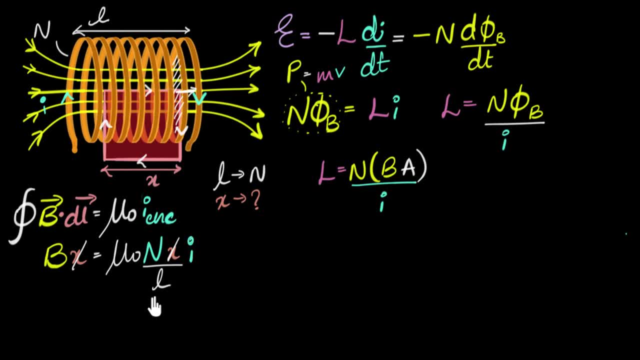 and deeply understand the derivation, And if you do that, you can pretty much derive all of these very quickly, so you don't have to remember stuff. All right, so that's how I do it, So now I can just plug this in. 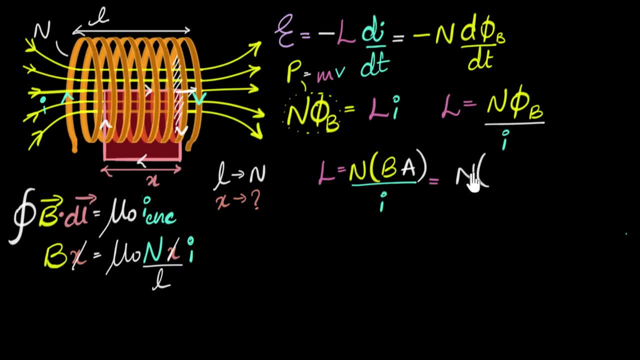 So if I plug in, I get n times. the expression for the magnetic field is: mu naught n I by L times. A divided by I and the I cancels out, and our final expression for L turns out to be: I pull that mu naught out. 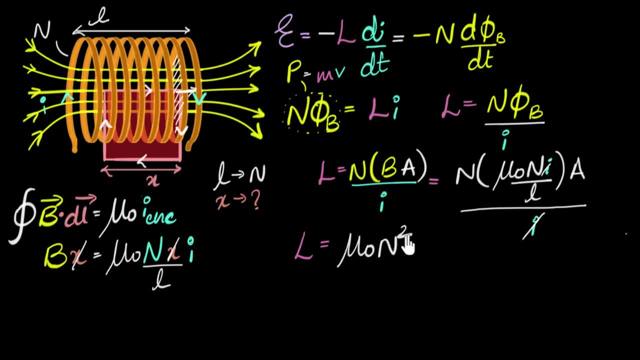 so it's gonna be mu naught n squared times A, where A represents the area of that loop divided by L, the length of the solenoid, And this is the expression. It'll only work for long solenoids. If you have very tiny solenoids, then the magnetic field is not gonna be useful. 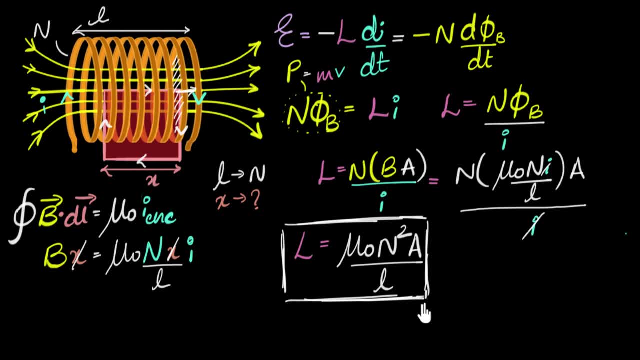 So if you have very tiny solenoids, then the magnetic field is not gonna be useful. So if you have very tiny solenoids, then the magnetic field is not gonna be useful. So if you have very tiny solenoids, then the magnetic field is not gonna be useful. 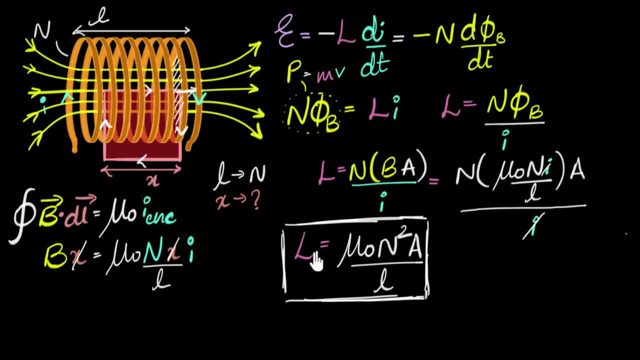 So what is this saying? Well, first of all, it's saying that it does. the self-inductance does not depend upon voltages or currents, but only on the geometry and on the material, just like capacitances or resistances. 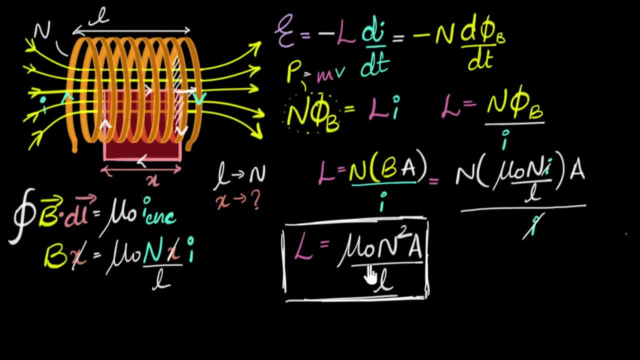 So that makes a lot of sense. But how does it depend on the geometry or the material? Well, let's look at geometry first. See, it says that if you have more turns, you get more self-inductance. How, why is that happening? 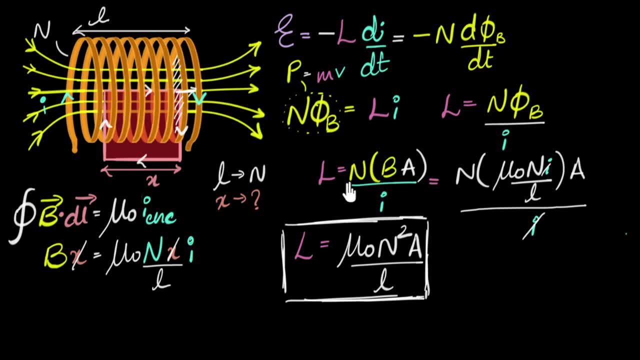 Because for more turns you tend to get more field for a given current. You also tend to get more flux for you know, more flux for a given current. So that's why more turns gives you more self-inductance. It says that more area also gives you more self-inductance. Why is that happening? Because with more area, you tend to get more flux for a given current. So that's how self-inductance tends to increase, And it says that if you increase the length, you tend to decrease the self-inductance. 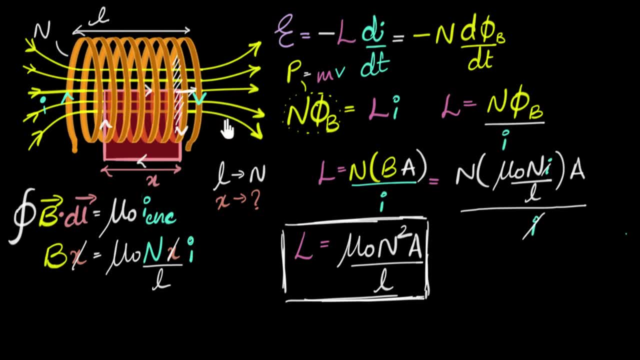 Why is that? Well, that comes from here. So if you tend to increase the length, then for a given current the field won't be much. If the coils go far away, the fields do not add up that much that nicely. 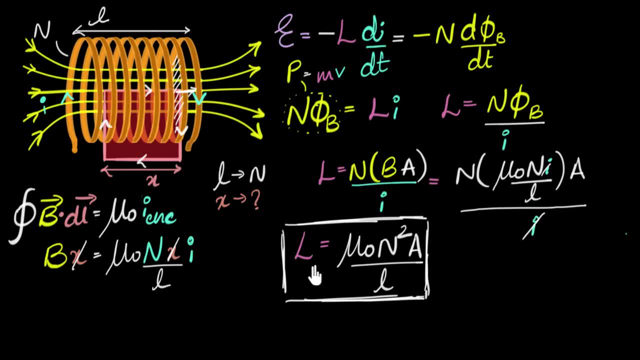 And so the fields will tend to reduce. So you tend to get less self-inductance, which means to have a higher self-inductance. not only it's important to have more turns, but you tightly, coil them tightly, make them short. 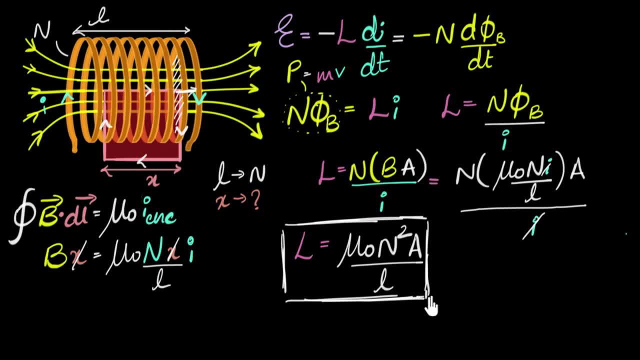 I mean, make the length shorter, you get more self-inductance. But how does it depend upon material? So it doesn't depend upon the material of the wire, but depends upon what is wrapped around. See if it's wrapped around air. 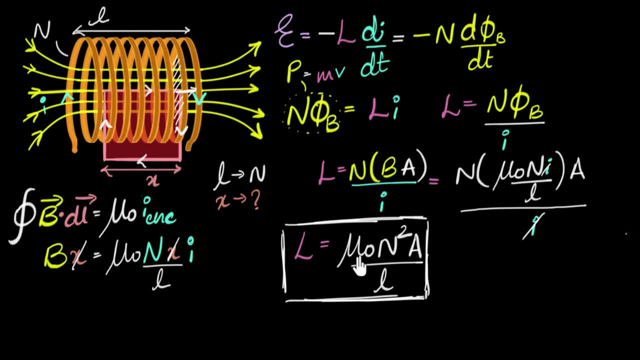 then you use mu naught permeability of air or vacuum, But say you wrap it around some kind of a ferromagnet, then the permeability of a ferromagnet is much, much higher than that of the air. So then the value will not be mu naught.